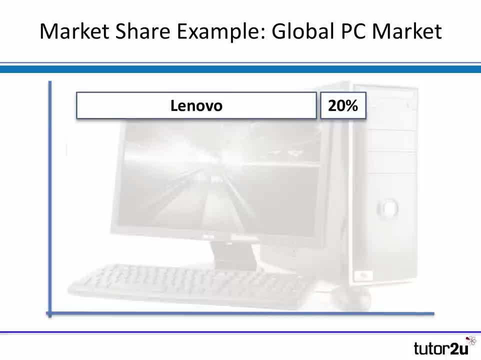 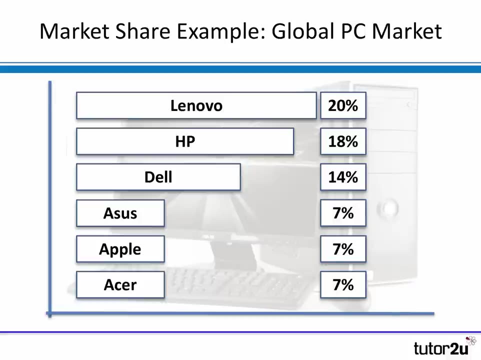 manufacturer and seller of PCs globally is Lenovo, a Chinese-based firm who have 20% of the global market in 2015.. And when you look at the remaining or the other leading players in the market, you can see how their market share is lower than Lenovo, HP, almost as large at 18% of the market. 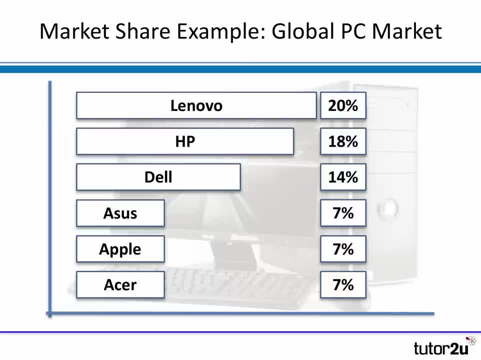 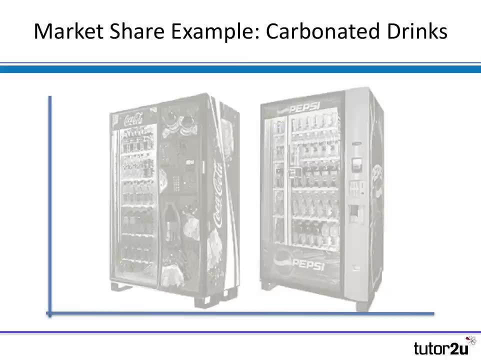 Dell at 14%, And then three manufacturers of personal computers- Asus, Apple and Acer- have 7% of the global market each. Let's take a look at one more example and you'll see some different types of market share information here. So here we're looking at the global market for what's known as carbonated drinks. 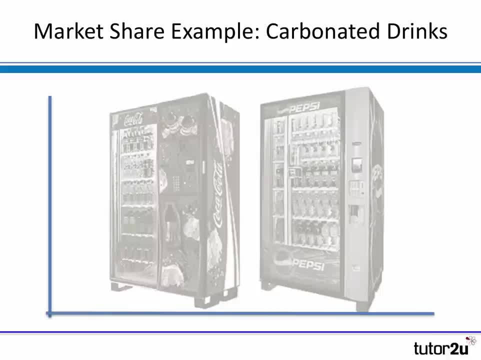 Cans of Coke and Pepsi. Who do you think has the largest market share? I bet most of you would guess that it's Coca-Cola. In fact, they have a whole range of different brands, don't they? But in total they have just under half or 49%. 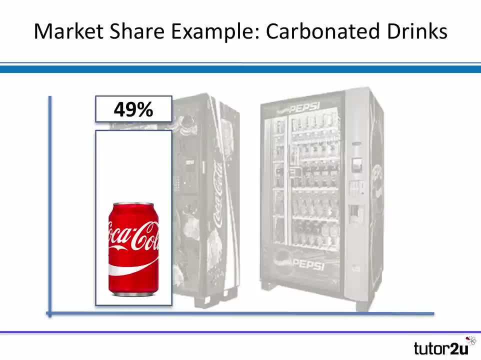 of the total volumes shipped in carbonated drinks globally, Five out of ten are Coca-Cola or Coca-Cola brands. Pepsi has a market share significantly lower than Coca-Cola globally at 20%, which means together the two of them account for about 70% of the global market, which means that the rest. 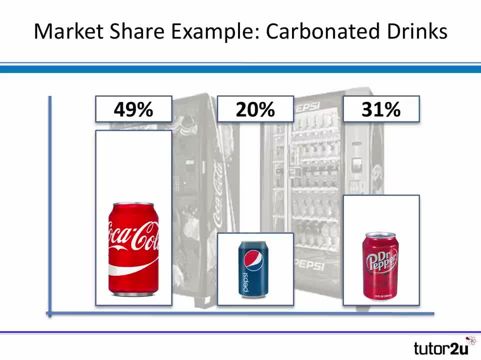 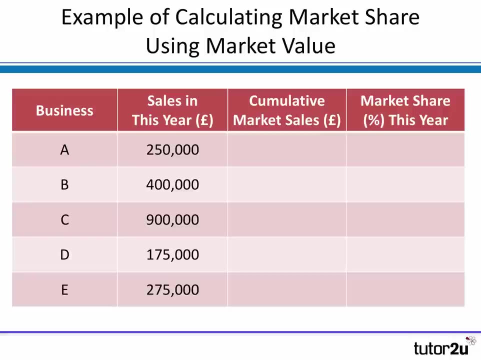 the likes of Dr Pepper and others, are fighting for their share, which is 31%, But that, by the way, is the data for 2015,. the billions of units shipped in 2015.. Now, when you get some information on markets and market size, if you're required to calculate, 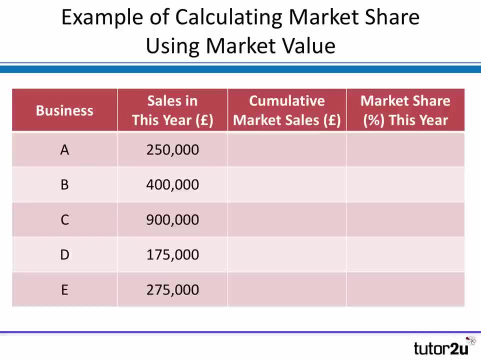 market share. what you need to be looking for is what is the total value of the market? So say, for example, you've got a table like this and you are asked to calculate market share, the first thing you need to do is to calculate the total. 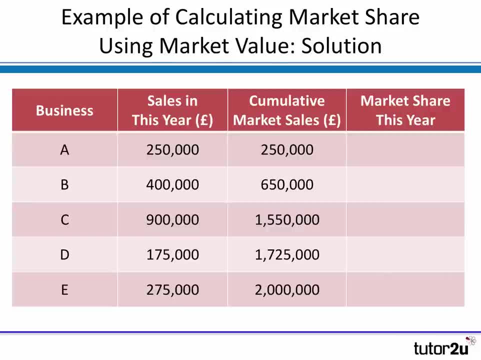 size of the market before you start to do any calculations. So if we have five businesses here- A, B, C, D and E- they each have separate sales ranging from what's the lowest, 175 company D, up to 900,000 for business C.